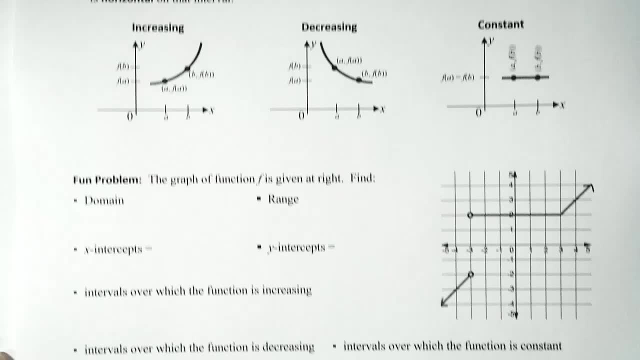 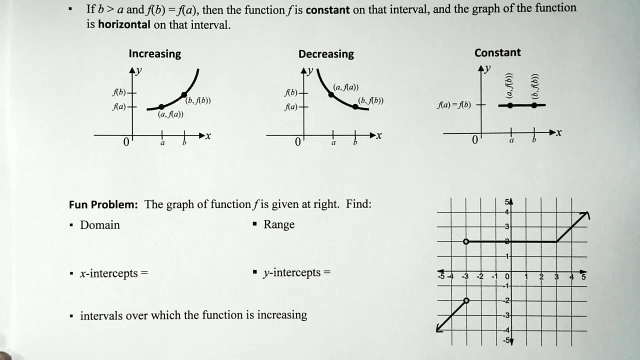 Just answer them. No one's going to know which one you answered first. Okay, so I'll just do it and send my order. Okay, domain. So, uh, from the beginning the semester we we had said that the domain is given by the set of all the input value or all the. 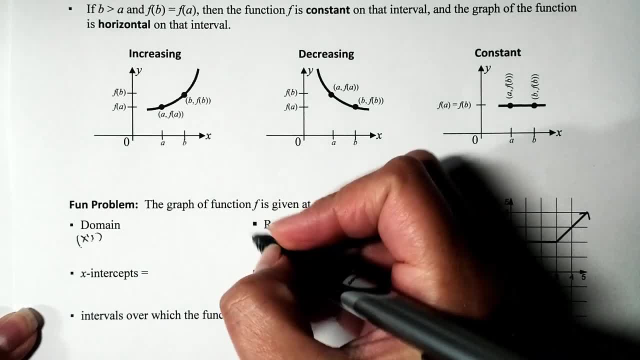 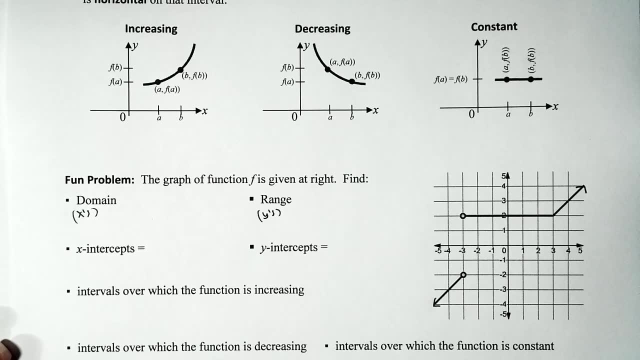 x values. The range is all the output values or the y's. So from this graph, what is the domain? So I want all the x's that are used to create this graph. So it looks like we have the x values that are smaller than negative 3.. So the interval is going to be from negative infinity to negative. 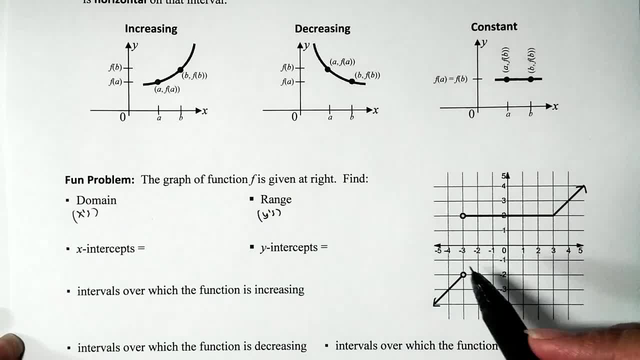 3, but I'm not quite sure if negative 3 is included. So instead of negative 3,, I'm going to definitely not include it here. I'm not sure if you can see it. Let me go ahead and zoom in. 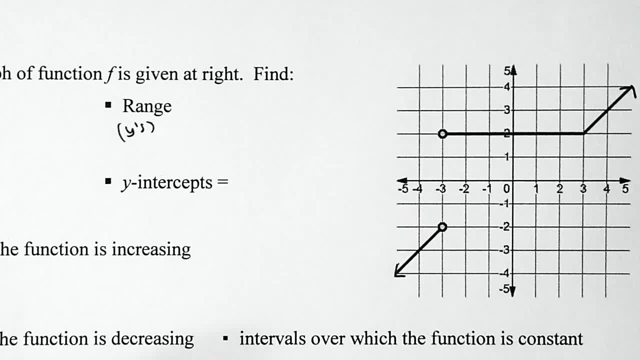 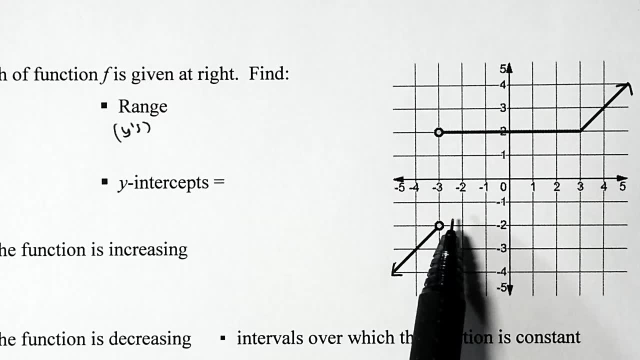 Okay, so in interval notation the domain is given by the set of all the input values or the x values that are used to create this graph. So I have all the negative numbers under negative 3.. So we have negative 4, negative 5, negative 6, negative 7.. At x equals negative 3,. uh, x equals negative, 3 is not. 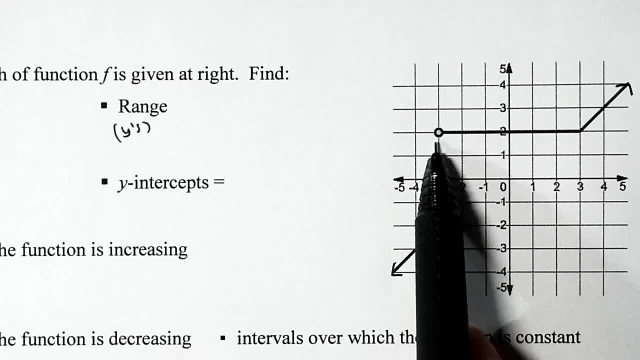 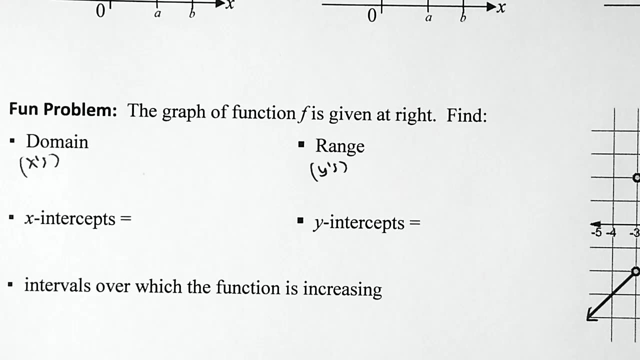 defined in this piece And I look up and we also have an open circle there. So actually the function is defined at x equals negative 3.. So in interval notation it's going to be from negative infinity to negative 3.. Let me go ahead and zoom out. So the domain: what are all the x values that are used to? 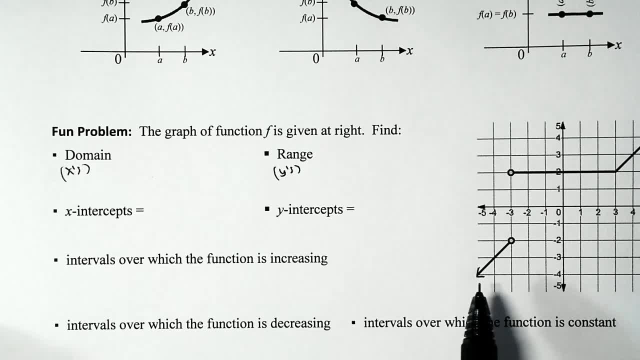 create this graph And in interval notation- because there's too many to spit out one by one- it's going to be given by negative infinity to negative 3, where negative 3 is excluded, And we also have more x values that are used to create the graph. We have x equals negative 3, and we also have 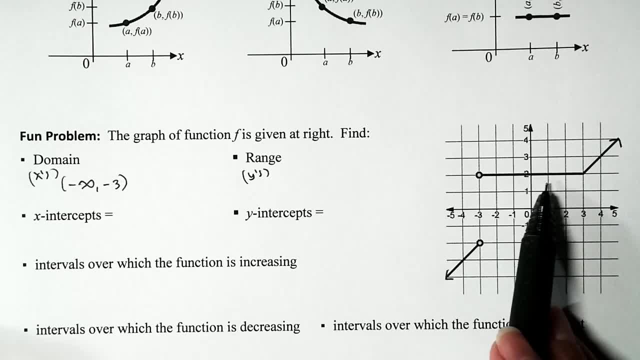 x equals negative 3, negative 2, negative 1,, 0,, 1,, 2,, 3,, 4, and all the way up. So pretty much we have the numbers that are less than negative 3 and the numbers that are bigger than negative 3.. So we're. 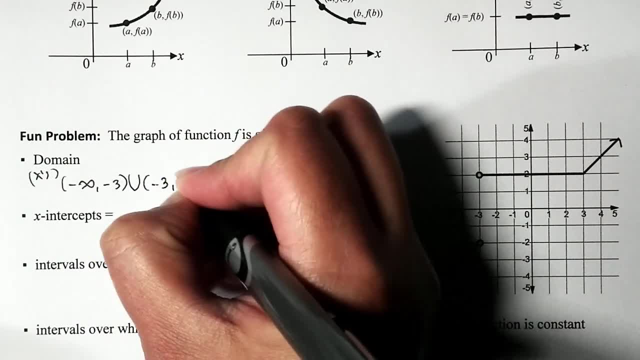 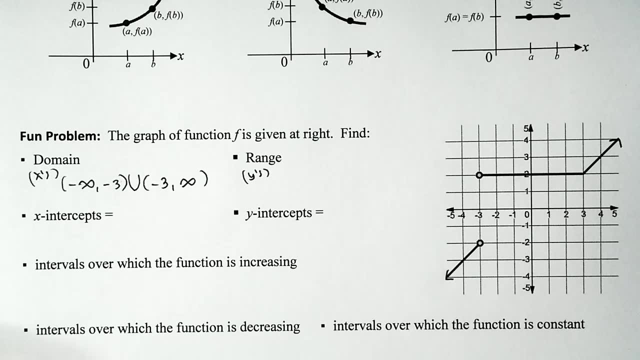 going to go ahead and throw a union symbol And it's going to be, uh, the interval from negative 3 to infinity. So, altogether, the domain, or the x values that are used to create this graph, is given by the interval from negative infinity to negative 3, where negative 3 is excluded, And we also have 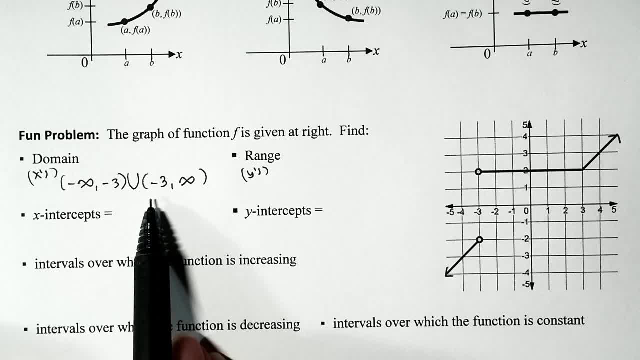 union symbol And it's going to be, uh, the interval from negative 3 to positive infinity, where, once again, negative 3 is excluded. Now, what about the y's? Uh, what are the output values, or what are the y values that are used to create this graph? So, from domain, since we go from left. 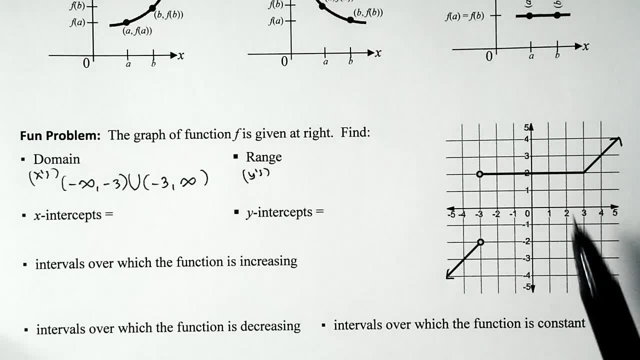 to right. on a similar note for range, we go bottom up. So what is the lowest uh value of this function or the lowest value of y? The lowest value of y is not negative 4, because this, this part, keeps extending forever and ever. So we're going to have all the negative y values. 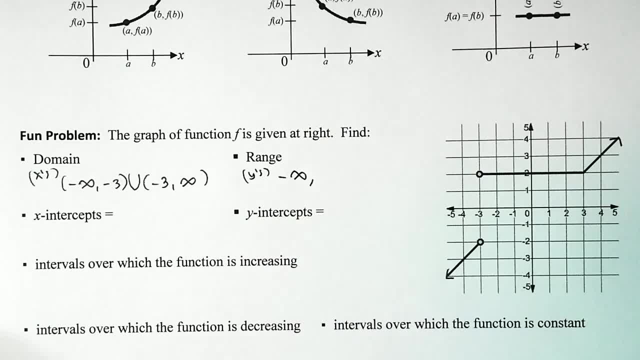 So it's going to be from negative infinity to what is the highest value of y. So let me go ahead, take out my special effect. I'm going to trace this curve And it looks like we have negative 4, negative 3,, negative 2.. And we take a little break, okay, So let's go ahead and write that. 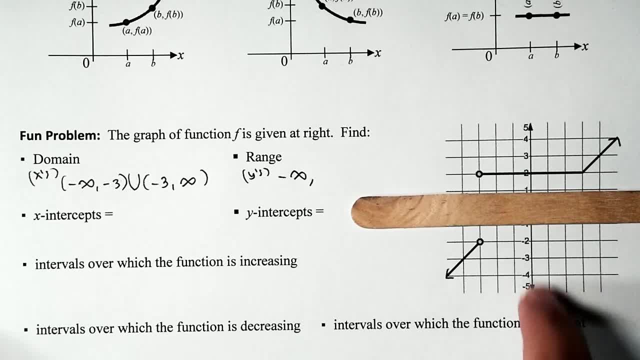 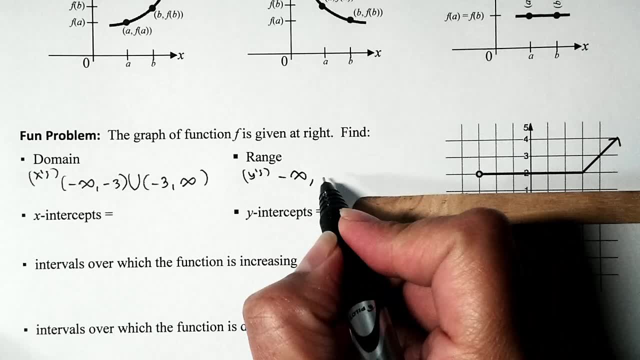 first interval. So all the y's, the lowest y to the highest y. So it's we have, we're coming from the negative side, So it's going to be from negative infinity to negative y, So we're going to negative 2.. And uh, this point is: uh is not there because of the open circle, So negative 2. 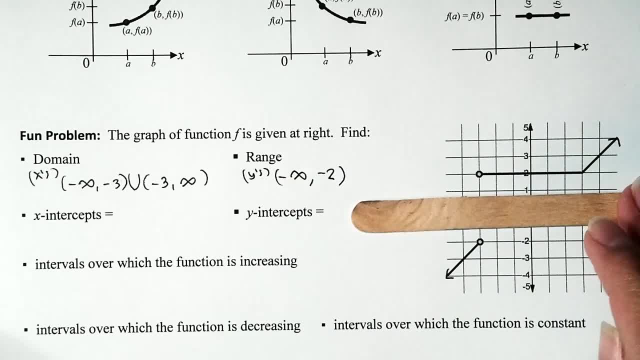 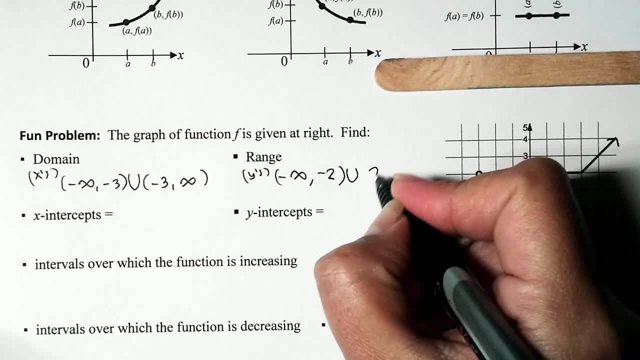 will be excluded. And then we have more y's that are used to create this graph. So we have y equals 2.. So we have union: y equals 2, until where do we stop? We have y equals 3.. We have y equals 4.. 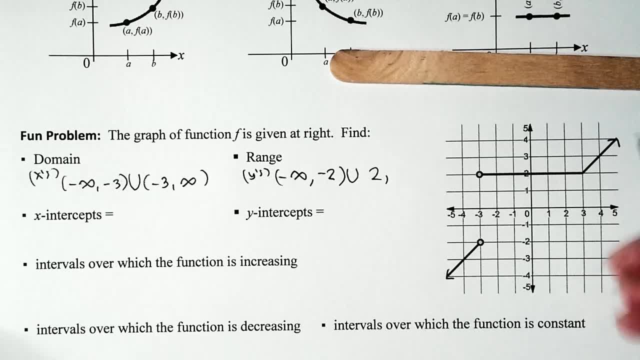 On graph, on the paper that we have, we have y equals 4.. But this bad boy keeps extending. So if we had the space, we would have y equals 6,, y equals 7, and so forth. So we're going. 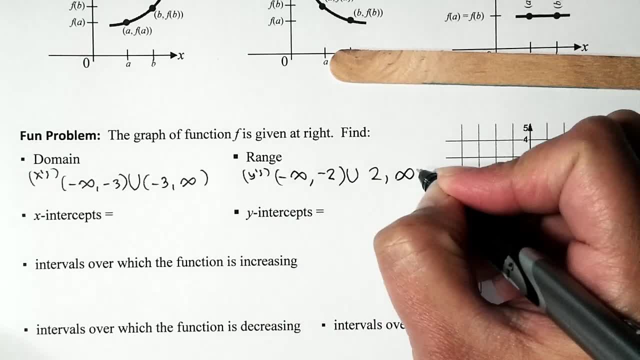 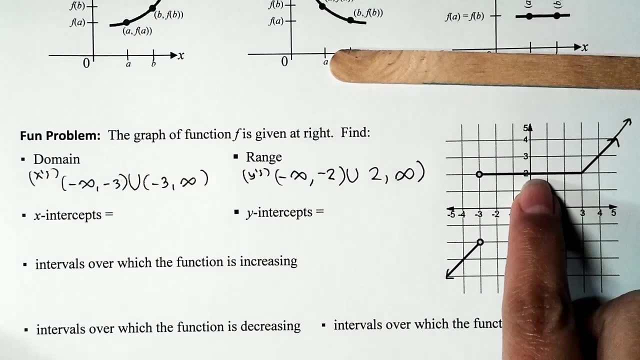 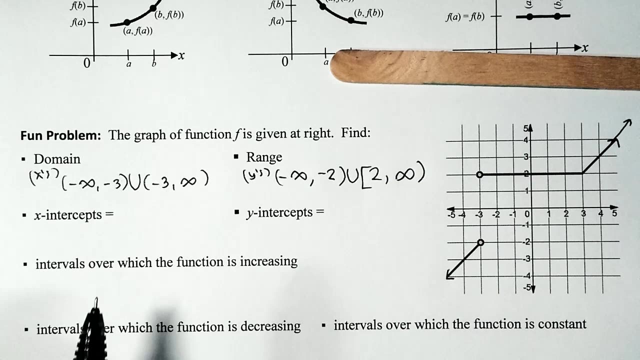 to have all the positive y. So we're going from 2 to infinity. The infinities are always- uh, always- get parentheses, because they don't represent specific numbers. And y equals 2, we have a y equals 2 on the graph, So it's going to go ahead. get a bracket, Okay, x and y intercepts X. 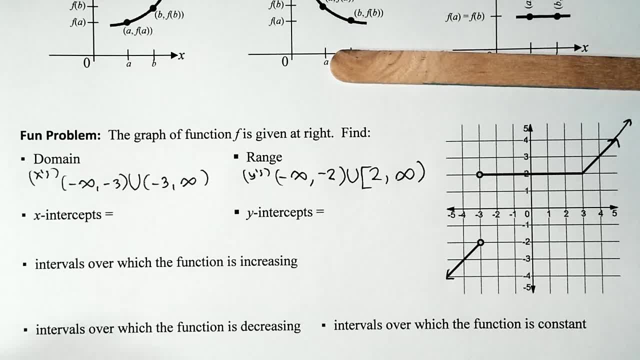 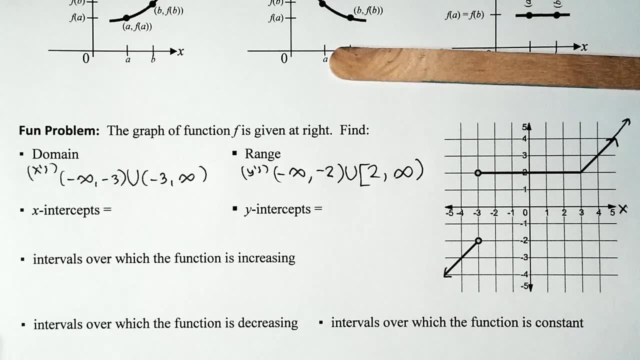 intercept point where the line intercepts the x-axis. So I'm going to go ahead, look at the graph and I want to know where does the graph intercept the x-axis? And uh, that's a lie because, as you can see, this graph does not intercept the x-axis. So there is there there. 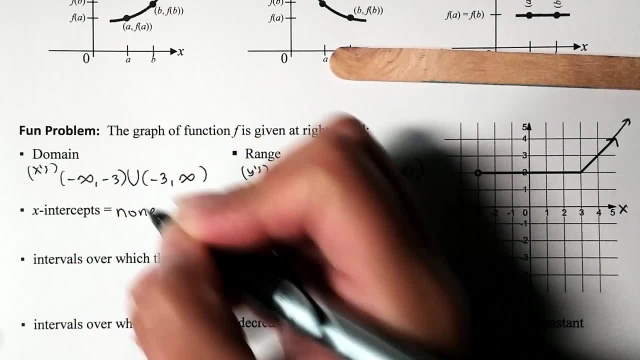 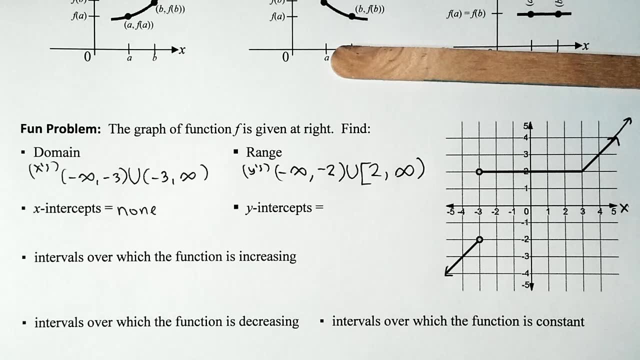 aren't any. So if you can do me a favor, write uh, any form of none or something to let me know that you just didn't know how to answer. Y intercept, uh, what is that Point where the line or the 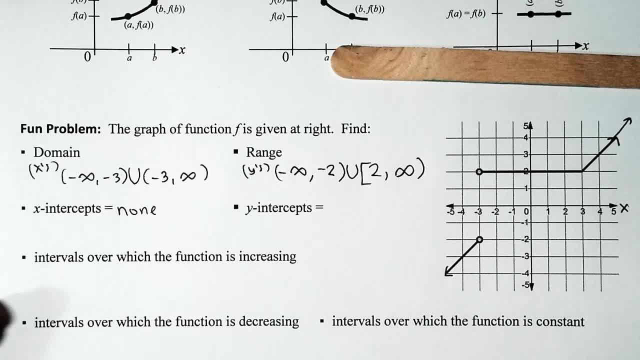 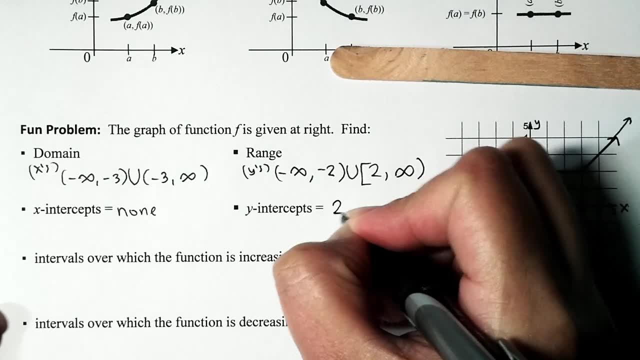 I'm sorry, point where the graph intercepts the y-axis. So in this case we have the vertical axis. So the graph intercepts the y-axis. So in this case we have the vertical axis. So in this case the y-axis is at 2.. So the y-intercept is at 2.. Okay, so fantastic, We answered the first 4. 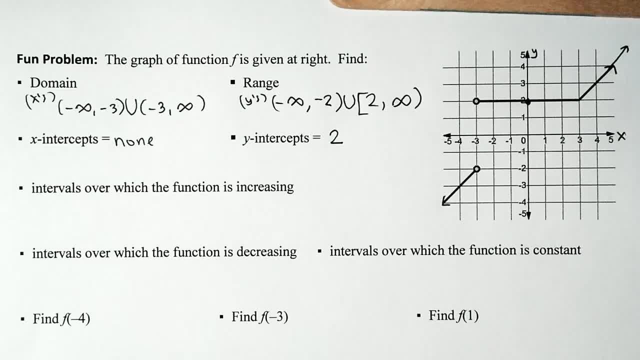 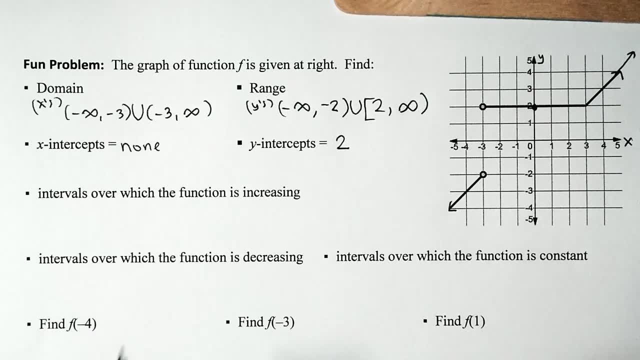 problems, Let's go ahead and knock out the remaining. If I know how to count, I believe 6.. Okay, the next 3, we're going to go ahead and answer them together. Okay, so we want to identify the intervals where the function is increasing, decreasing or constant. Now you can answer them. 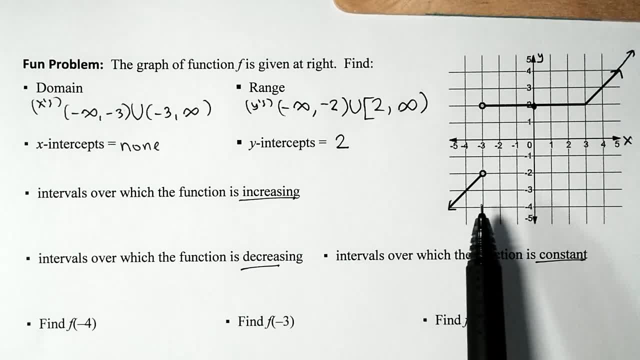 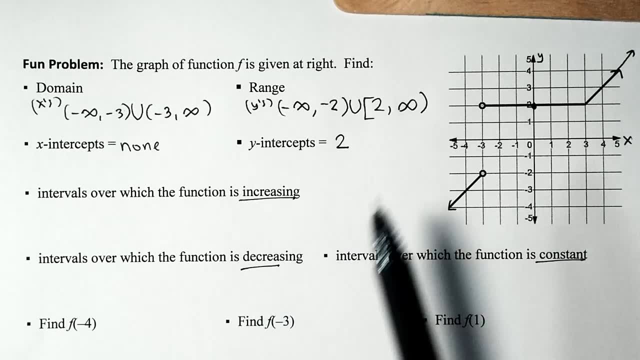 in order, but but for me it's a little bit easier just to read this graph from left to right. If the function is increasing, we put it right there, If the function is decreasing, we put it right there, And if the function is constant, we put it right there. So as we trace this graph from 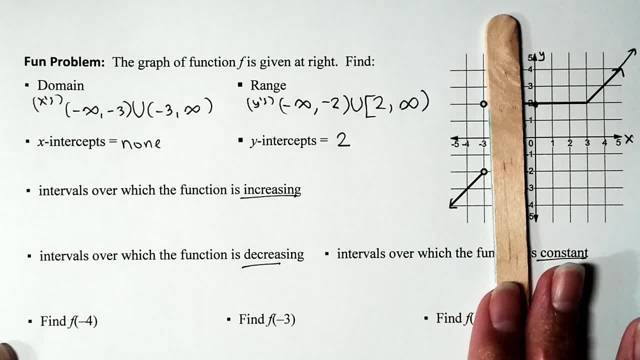 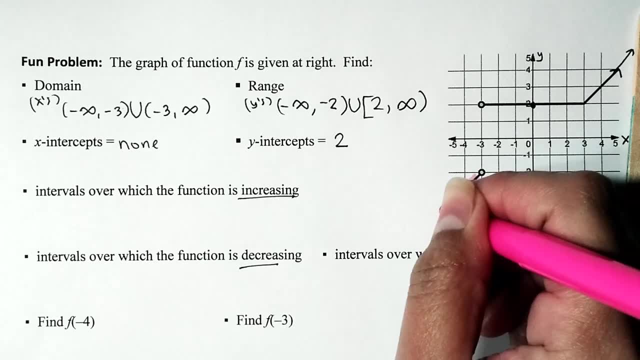 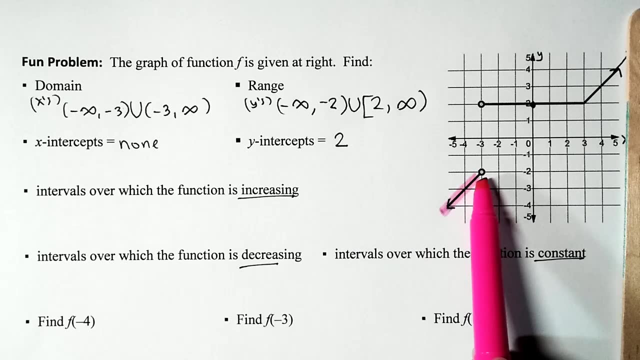 left to right. look at my special effect. Looks like we're going up. Okay, so the function is going to is increasing from this x value all the way to that x value. The x values are the numbers that are smaller than negative 3. So it's from negative infinity to negative 3.. This point is: 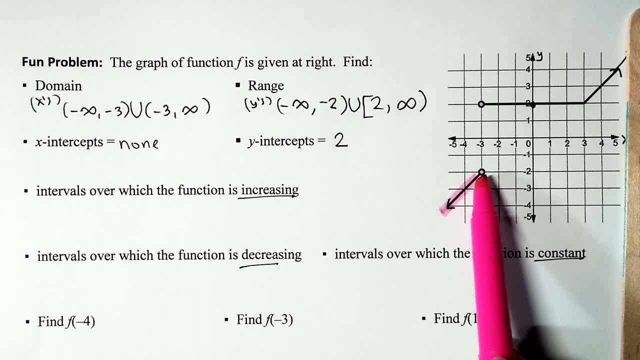 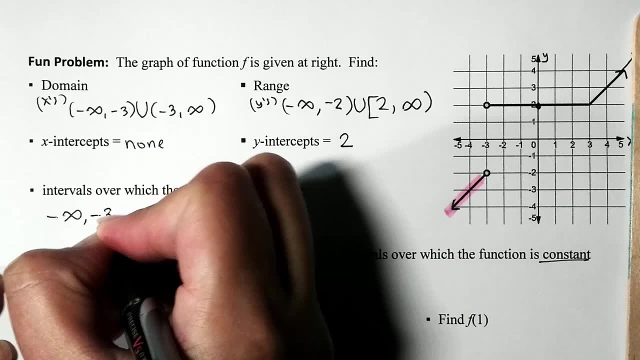 out. So it's going to be um from negative infinity to negative 3, where negative 3 is excluded. So let me go ahead, pencil that in: So negative infinity to negative 3.. I understand that this is not a pencil, That's just how I speak. 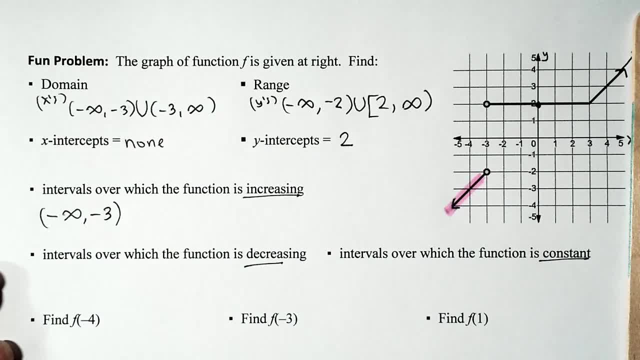 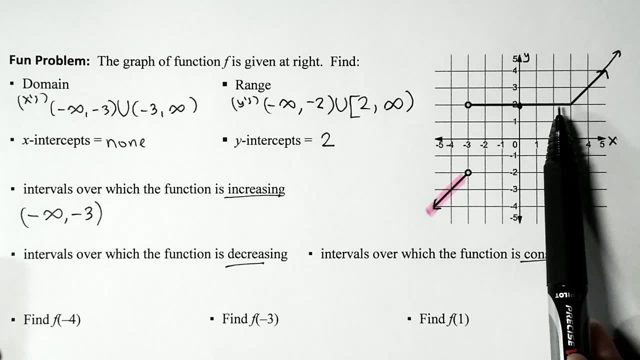 Okay, so negative 3 is excluded. Okay, we keep, uh, looking at this graph, We keep tracing it, Um, we, we zoom over here and then it is flat or constant, as some of you may say, And we want to tell the reader that the graph or the 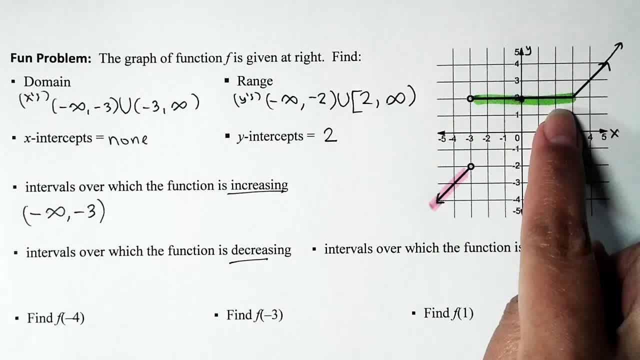 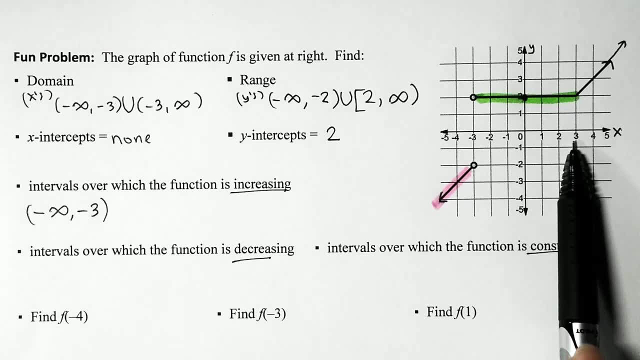 the graph or the function is constant from this x value to that x value. At this point, the value of x is negative 3.. At this point, the value of x is positive 3.. So we want to tell the reader that the 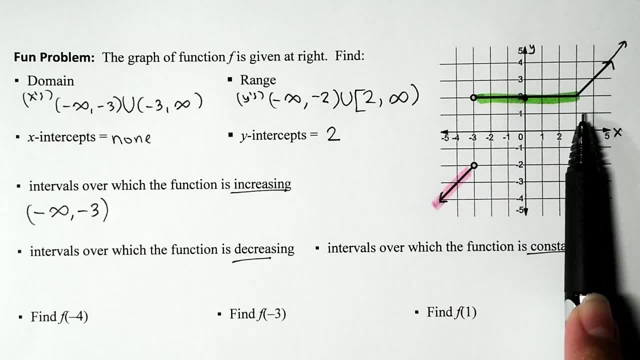 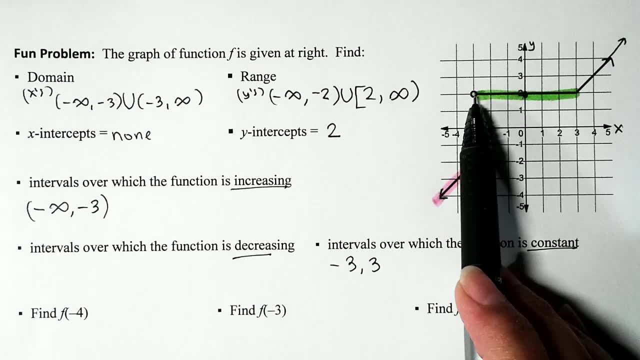 function is constant. from x equals negative 3 to positive 3.. So let's go ahead, put that in interval notation. So it's going to be the interval from negative 3 to positive 3.. This point is not graphed, It is fake graph because we have an open circle. So we're going to put parentheses at negative 3.. 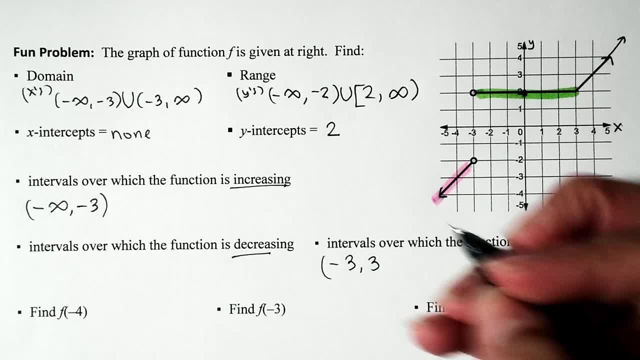 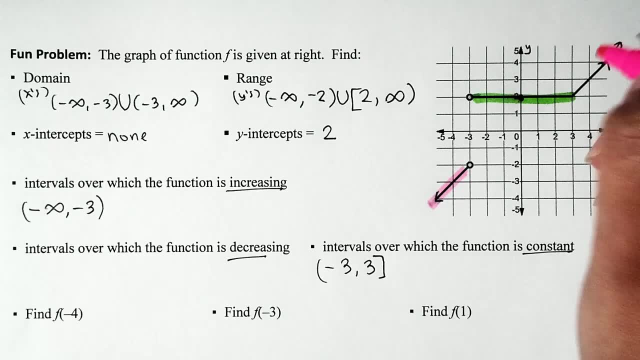 And then this point is graphed, So we're going to go ahead, include that. Okay. so, uh, if we keep tracing this graph, uh, after 3, then we are going up or it is increasing, So let's go ahead and do. 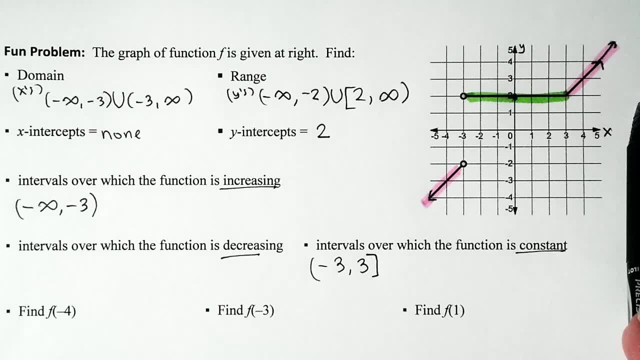 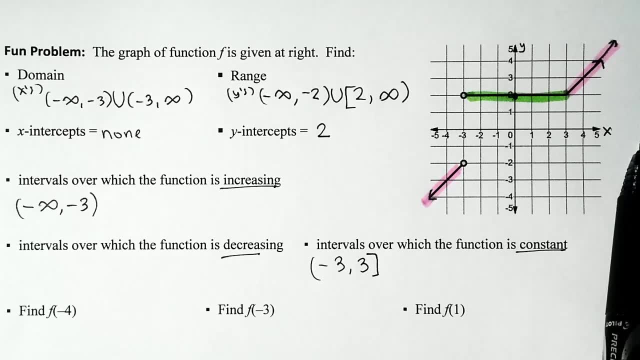 this Okay. so it's increasing from this x value to that at to that x value. Sorry for my pause. So we're increasing from x equals 3, and we're getting all the positive numbers. So it's going to be from 3 to infinity. 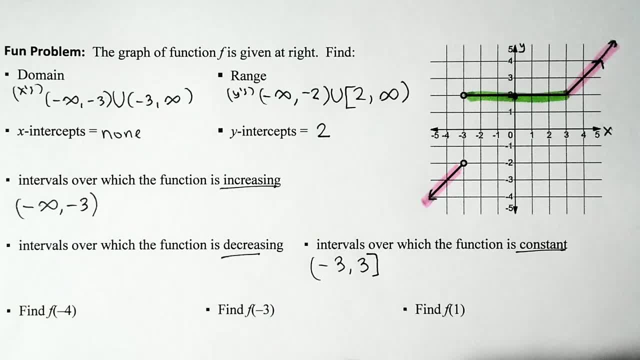 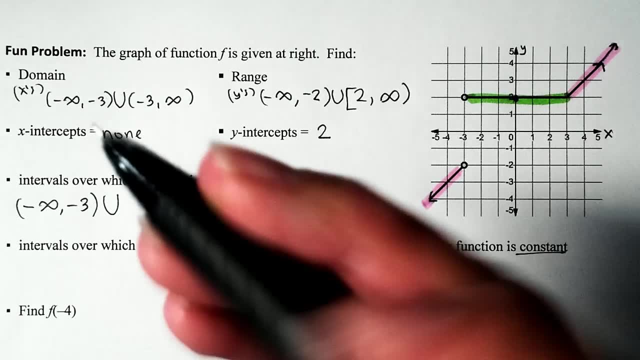 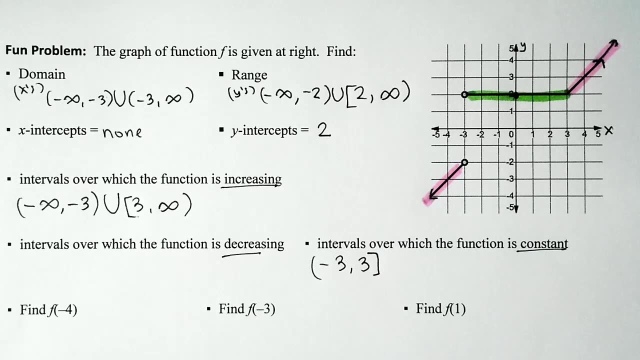 We already have an interval, uh, in the increasing, So we're going to go ahead, put the union symbol. So, uh, once again, the function is also increasing from x equals 3 to infinity, or the interval from 3 to infinity, Fantastic. So, uh, I think we're done tracing the the graph. Uh, there's not a. 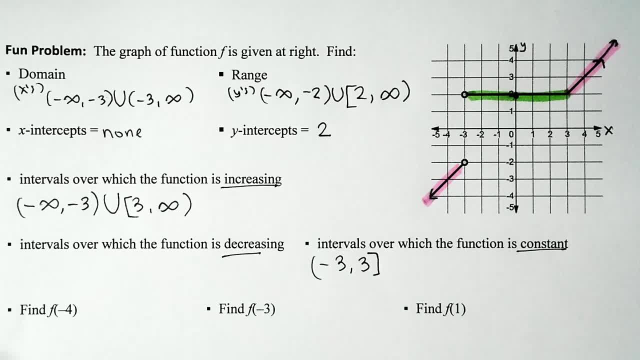 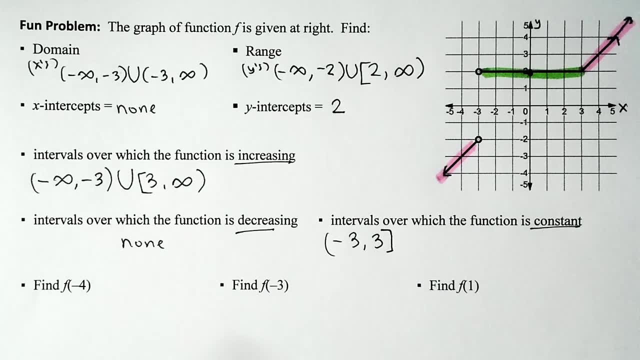 uh, an interval where the function is decreasing. So same speech. If it doesn't apply, just put none. For the grand finale, let's go ahead. Evaluate this function at negative 4,, negative 3, and 1.. So, f of negative 4,, what is the value of this function? 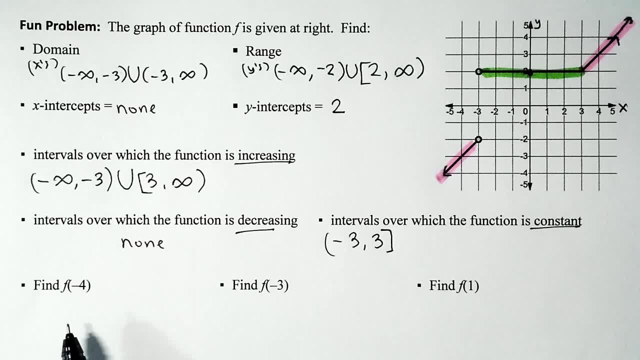 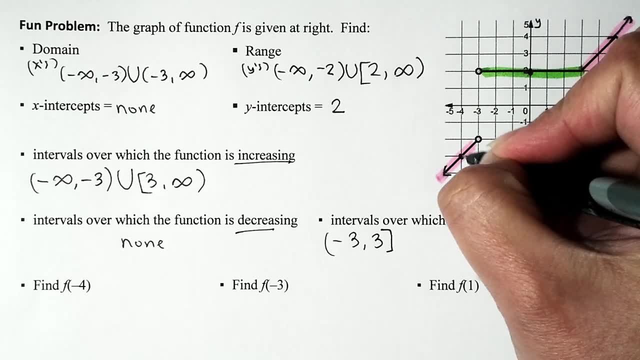 when the input equals negative 4?? So this is how I do it: I pretty much locate negative 4 on the x-axis and then I go up or down until I hit my mark. So in this case we go down, and at this point let me go ahead label. 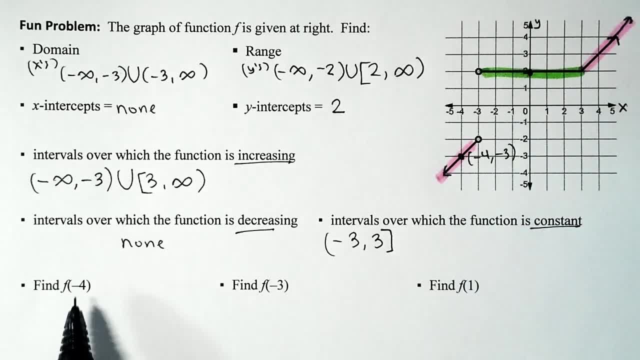 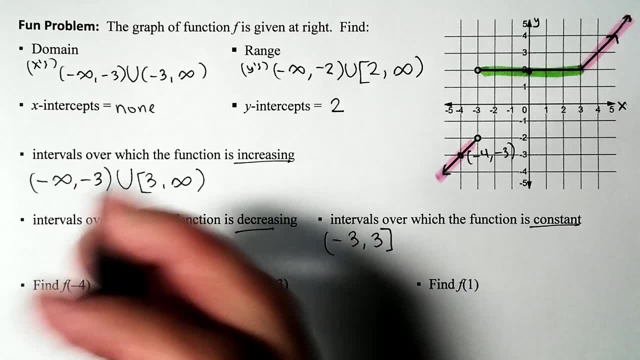 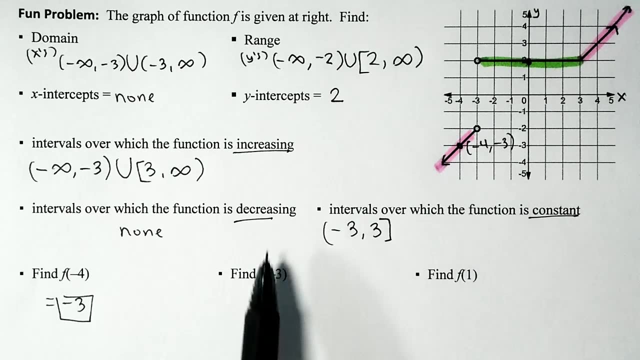 the coordinate, It's negative 4, negative 3.. So f of negative 4, when the input is negative 4, the output is negative 3, or the value of the function. So in this case, f of negative 4, with confidence equals negative 3.. For the almost grand finale, f of negative 3.. 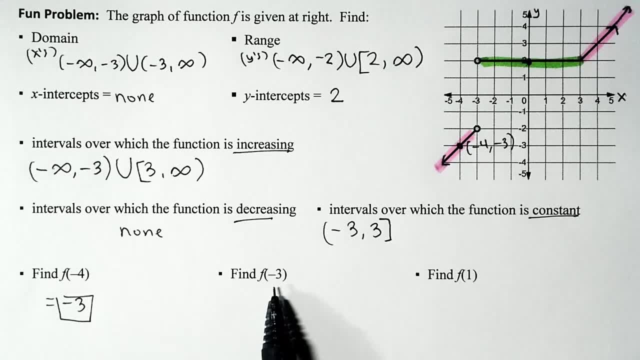 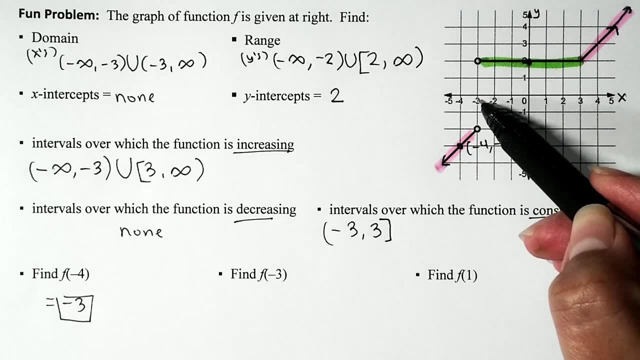 So we want to evaluate this function at negative 3.. So when the input is negative 3, what is the output? So I'm going to locate um negative 3 on the x-axis and then I'll go up or down until I hit my graph. 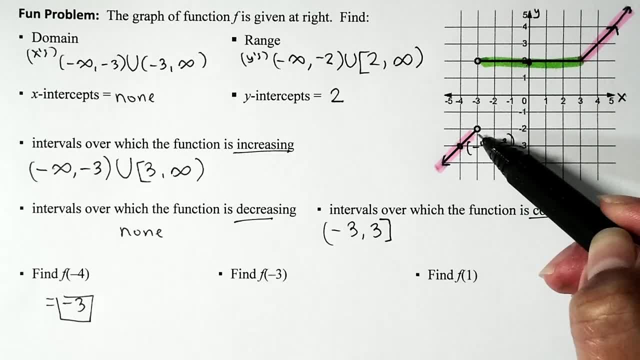 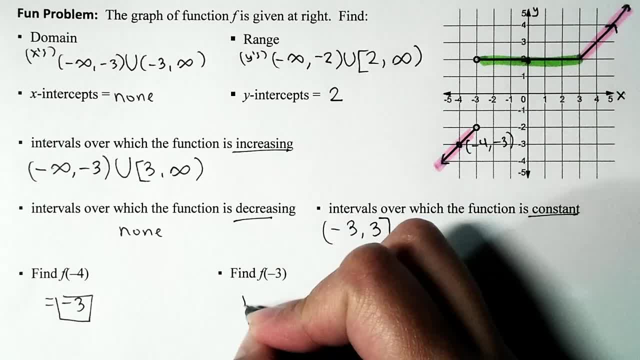 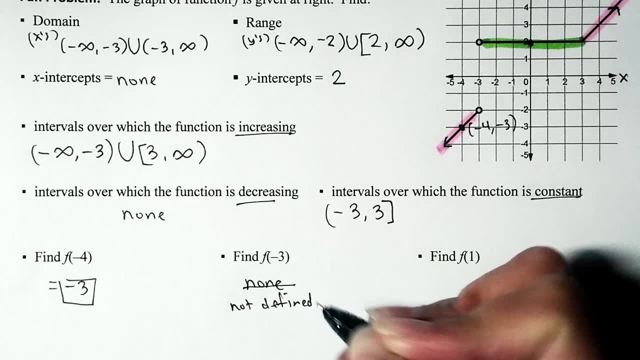 So, um, the function is not defined at negative 3.. So we're just going to say none, Oh, not defined, Sorry. So the function is not defined at f of negative 3, but, um, the books don't write that, They'll just write undefined. 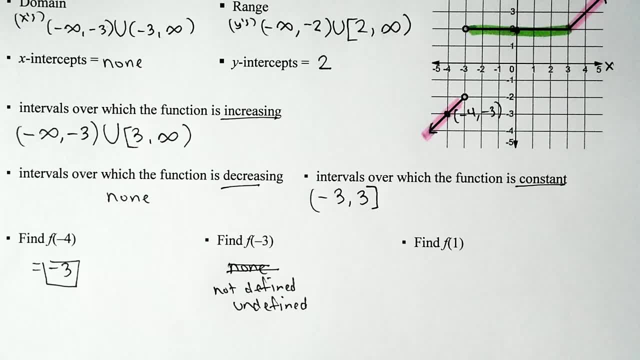 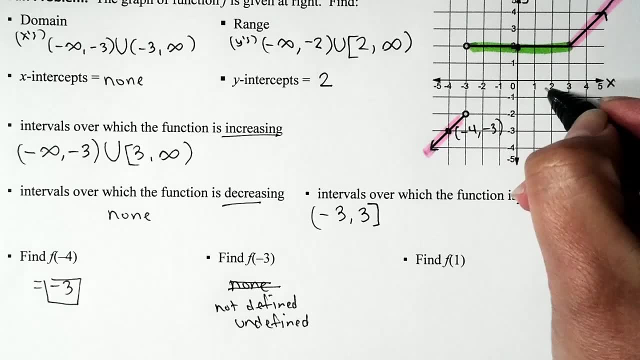 It's a. it's a personal choice. Okay, So f of 1.. So we want to evaluate that function at 1.. So, when the input is 1, what is the output? So, uh, let's go ahead and locate 1 on the x-axis and we'll go up or down until we hit our mark. 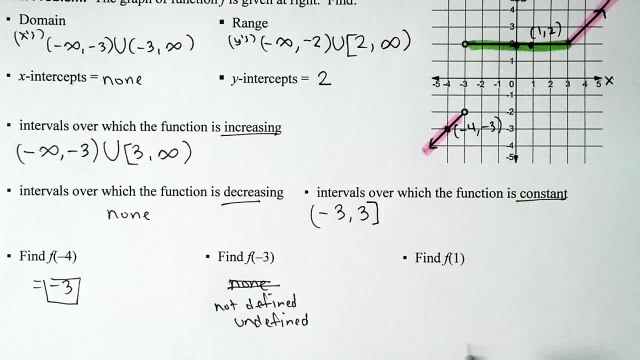 And at this point we are at 1, 2.. So the model of this story is: f of 1 is 2.. The value of this function at 1 is 2.. Okay, so I think we hit all these problems, so we're good to go. Thanks, guys.